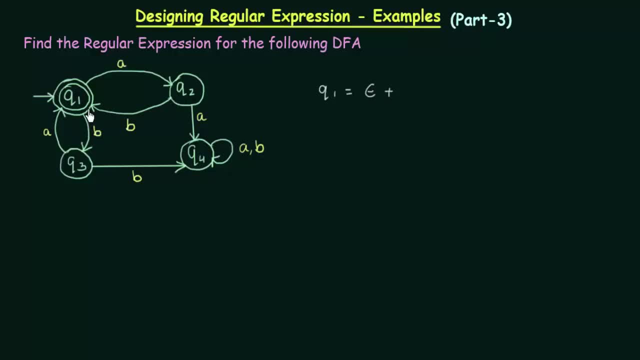 and here we see that from Q2 there is an incoming transition with input B, So we can write Q2B Plus, and then from Q3 also there is incoming transition to Q1 with input A, So I have to write Q3A and then there are no more incoming transitions. 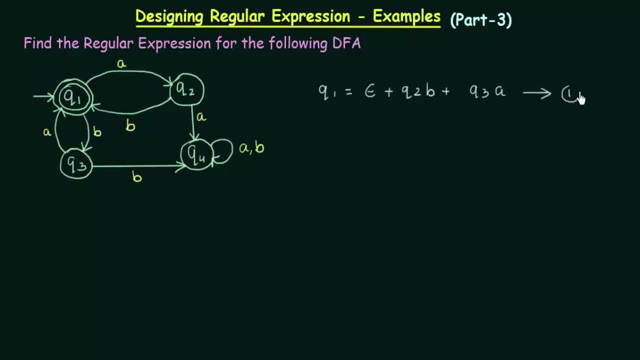 So this is the equation for Q1, and let me call it equation number one. Now let's do the same thing for equation number two, that is, for Q2.. So in Q2 we see that there is only one incoming transition, that is, from Q1, with input A. 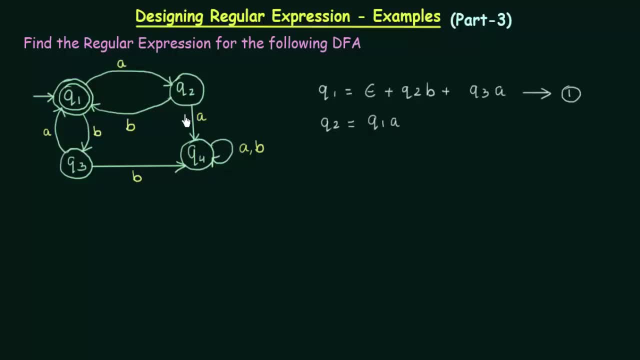 So we can write it as Q1B And there are no more incoming transitions to Q2.. So this is equation number two. Now let's do the same thing for Q3.. So for Q3 also, we see that there is only one incoming transition, that is, from Q1 to Q3 with input B. 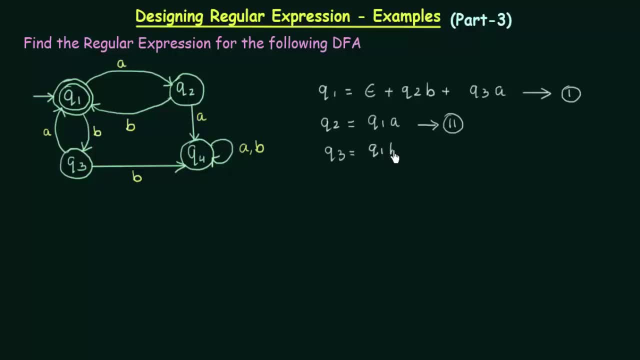 So, since it is coming from Q1, I will write Q1 and input is B, So this one. let me call it equation number three And let's do the same thing for Q4.. So in Q4 we see that there are incoming transitions from Q2, Q3 and also from Q4.. 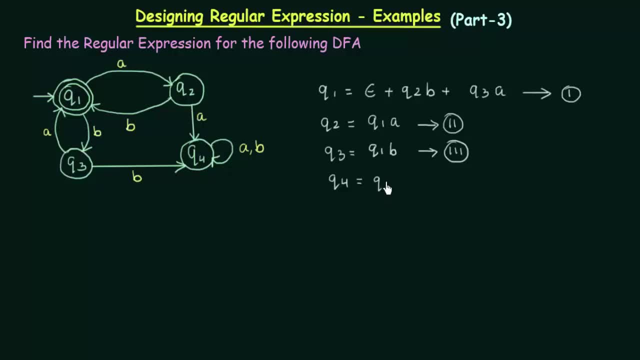 So let me first write the one for Q2.. Q2: it comes with input A plus. from Q3 it is coming with input B, Q3, B And for Q4 it is coming with both input A and B, So we have to write Q4 with input A plus. 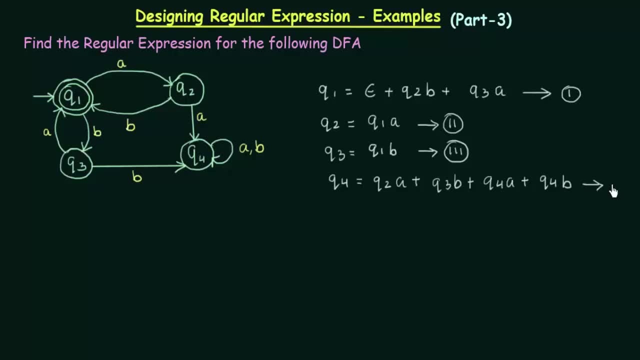 Q4 with input B. So this is equation number four. Okay, so now we have written the equations for all the states. Now let us try to take this final state and try to simplify it. Final state is Q1.. So that is equation number one. 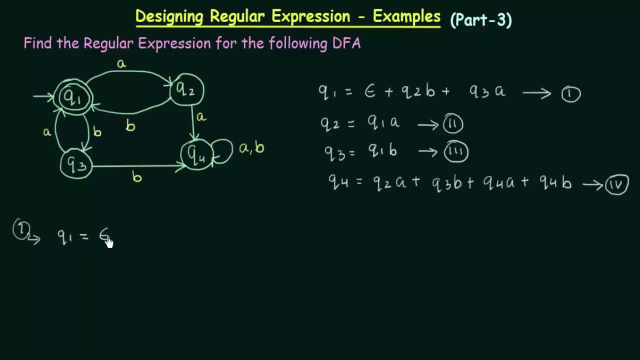 I take, and that is Q1.. And what is Q1? Epsilon plus Q2B plus Q3A. Now we see that we have Q2 and Q3 over here And this Q2 and Q3 values can be substituted from equations two and three. 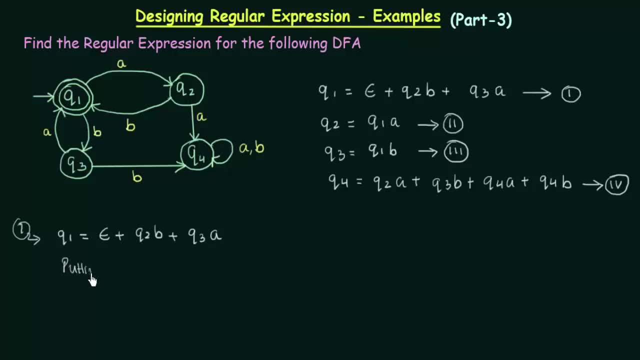 So let me put the values, So let me write here, Putting values of Q2 and Q3 from equations two and three. So how can we write this? Q1 equal to this epsilon will be as it is, epsilon plus. 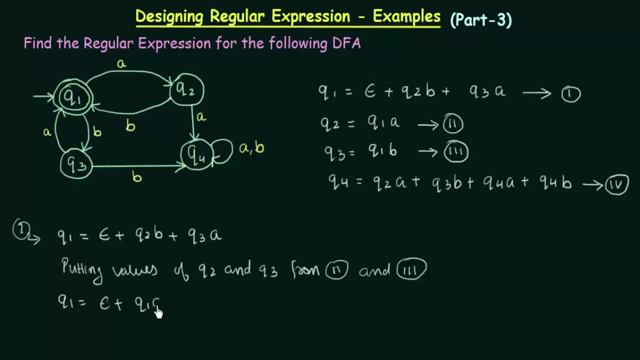 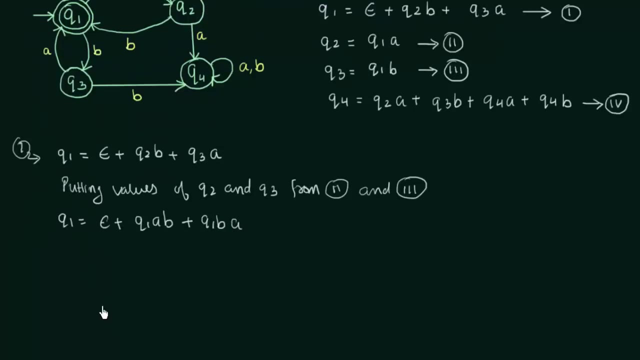 Now Q2 can be written as Q1A and this B can be written as B itself, plus Q3.. Q3 can be written as Q1B and this A- I will write it as A itself. Okay, so now we get this, and from here I see that I have Q1, Q1. 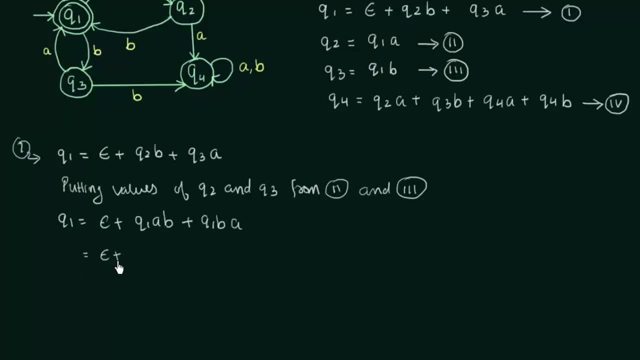 So I can take out Q1 common, So epsilon plus. let me take out Q1 common. So what do I get? I get AB plus BA. Now, if you observe this equation, Q1 equal to epsilon plus Q1, AB plus BA. 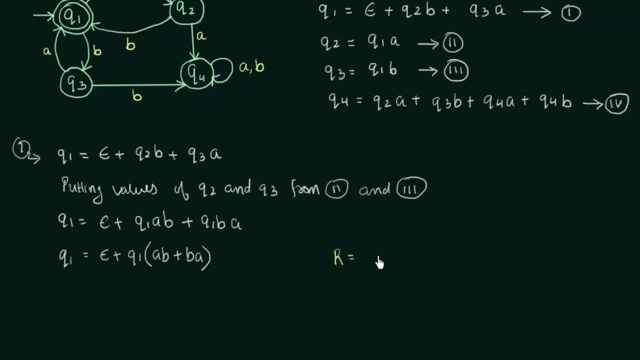 We can see that this equation is of the form R equal to Q plus RP, Where this Q1 is R and this epsilon is Q And Q1 is R, as we said, and this whole term over here this is P, So this can be written as R equal to QP, star by Arden's theorem. 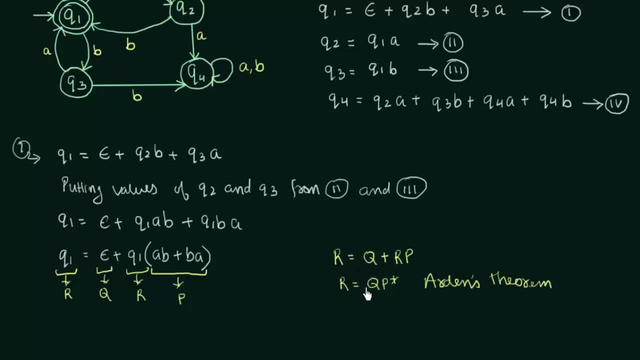 So whenever you have an equation of the form R equal to Q plus RP, it can be written as R equal to QP, star by Arden's theorem. So this is of that form, So let me write it in this form. 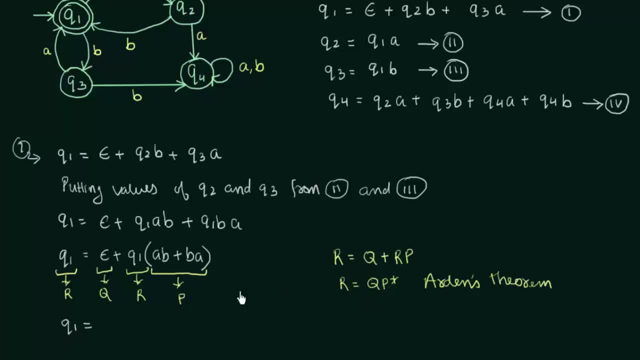 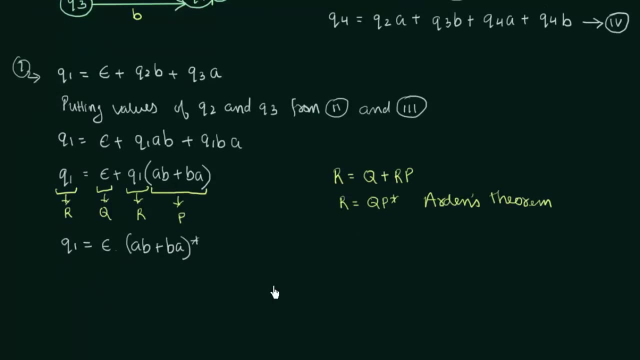 So R is Q1 and QP star, Q is epsilon and P star. This whole term is P AB plus BA star. So this is what we are getting And here we see that epsilon into this term. So we have also studied from our identities that epsilon into any regular expression. R is equal to R itself.